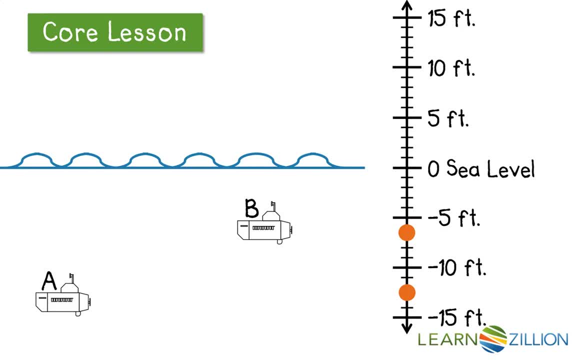 This is why absolute value is so important. Remember that absolute value refers to the distance from zero. In this example, submarine A has an absolute value of twelve and a half feet and submarine B has an absolute value of six and a half feet. 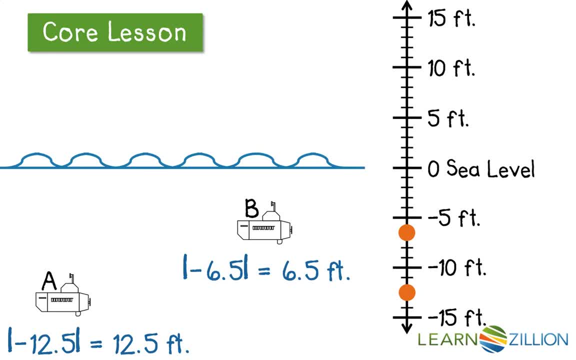 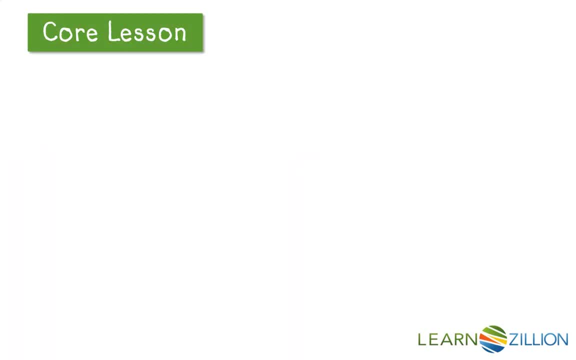 This shows that submarine A is deeper than submarine B because it is further from sea level. In the beginning of the lesson I asked: when could negative four and seventy-five hundredths be more than negative two and twenty-five hundredths? Here's an example that shows when this is possible. 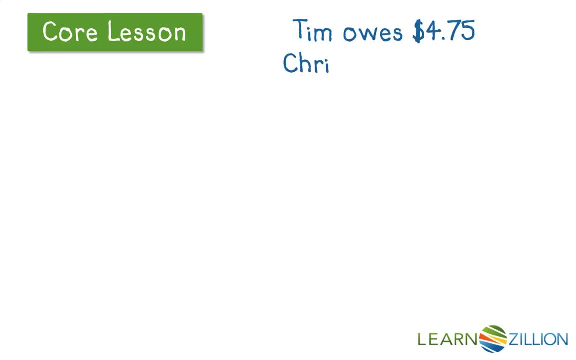 Tim owes his mom four dollars and seventy-five cents and Chris owes his mom two dollars and twenty-five cents. Now, who owes more money In this example when I place negative four and seventy-five hundredths on the number line, or negative four dollars and seventy-five cents? 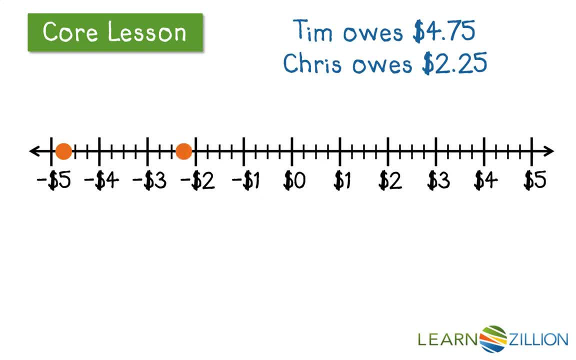 and I compare it or I find the relationship between that and Chris's value that he owes, which is two dollars and twenty-five cents. they're both in debt, but who has more debt and who has less debt? Well, the absolute value of negative four dollars and seventy-five cents is four dollars and seventy-five cents in debt. 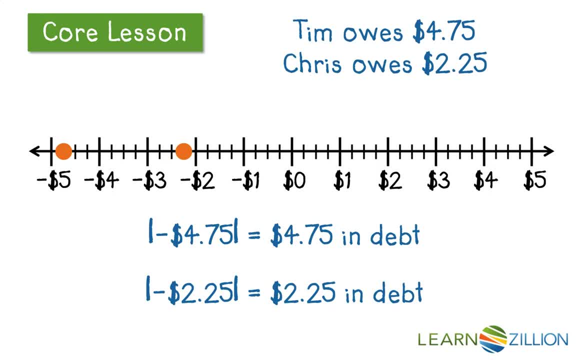 and the other value that Chris owes is negative two dollars and twenty-five cents. The absolute value of that is two dollars and twenty-five cents in debt. In this example, Tim owes more money than Chris, so in this example, the absolute value of negative four dollars and seventy-five cents is more than the absolute value of negative two dollars and twenty-five cents. 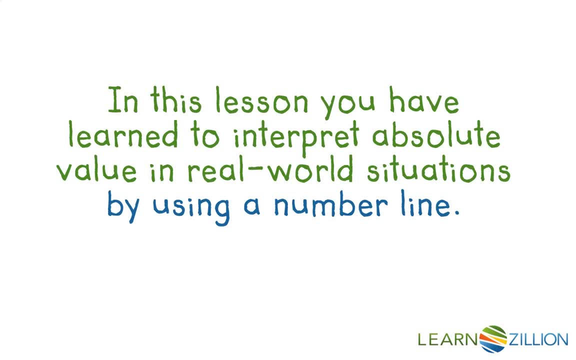 In this lesson, you have learned to interpret absolute value in real-world situations by using a number line. Thank you.